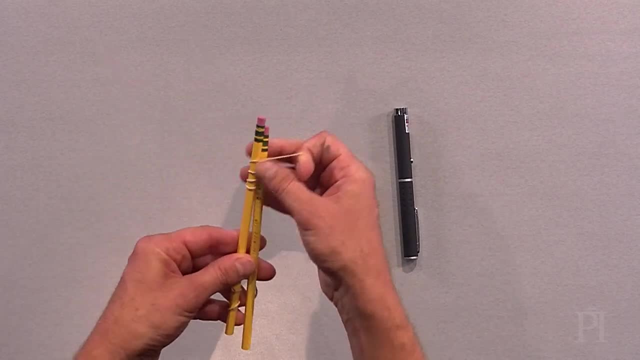 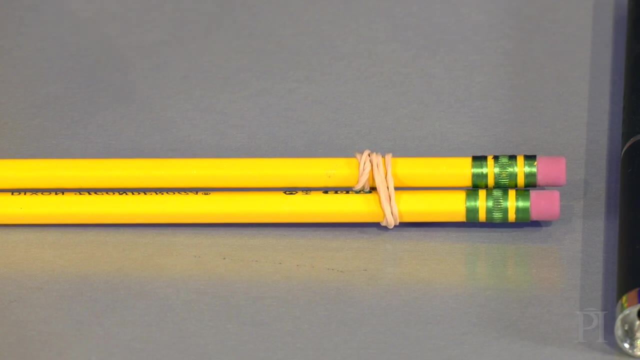 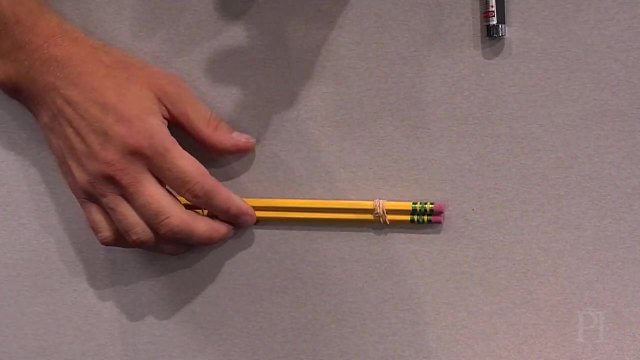 elastic bands around a second pencil again a couple of times. The elastic around just one of the pencils creates a small gap between them. It should be about a millimeter or two, but the exact size doesn't matter. Now hold the pencils horizontally, resting your arm on the table to. 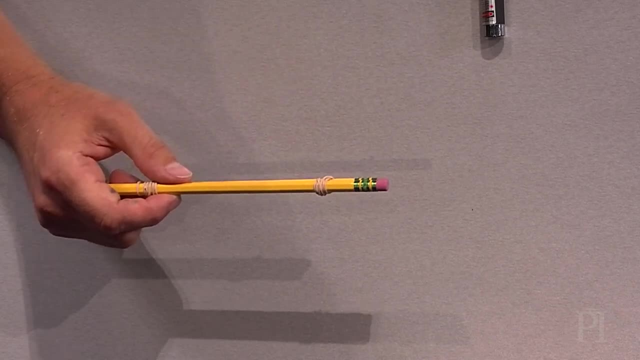 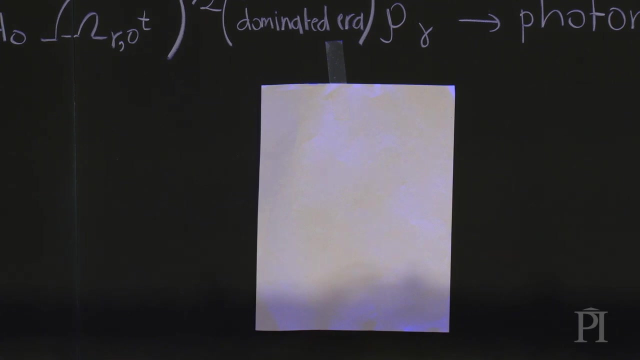 keep them still. Pick a spot that's a few meters away from a wall, ideally one that's white or some other light color. If you don't have a light color, you can use a light color. If you don't have a light colored wall, tape a white piece of paper to a wall. Put the laser right up to the pencil. so 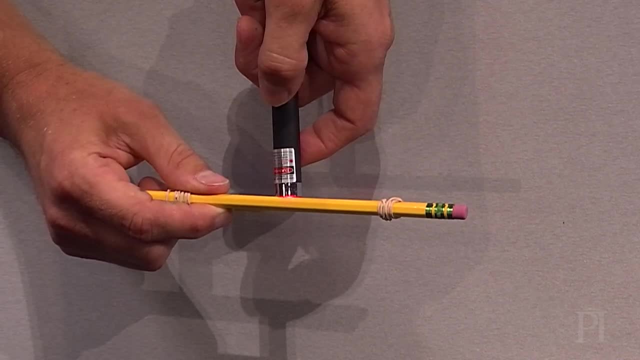 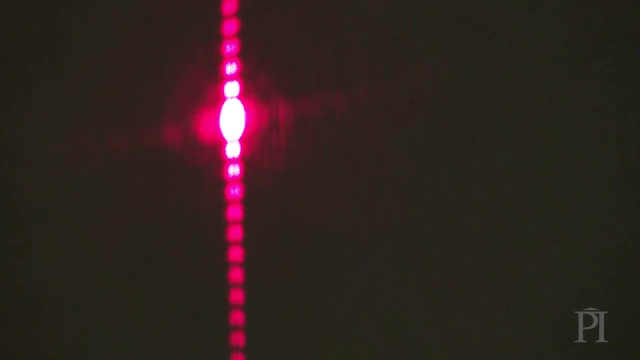 that it's touching and shines through the gap. Of course, make sure you take appropriate safety precautions when using the laser. A vertical diffraction pattern will appear on the wall. It's easy to see if the lights are off or even just dimmed. Rest your arm holding the laser on. 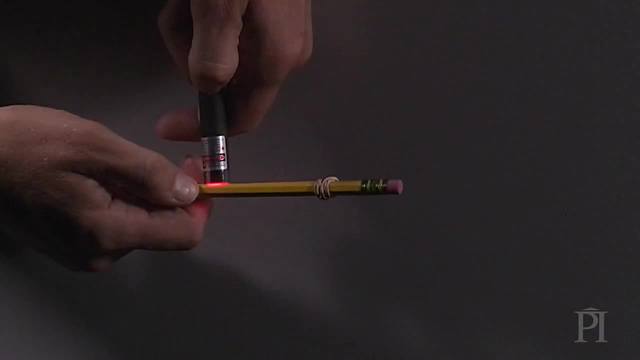 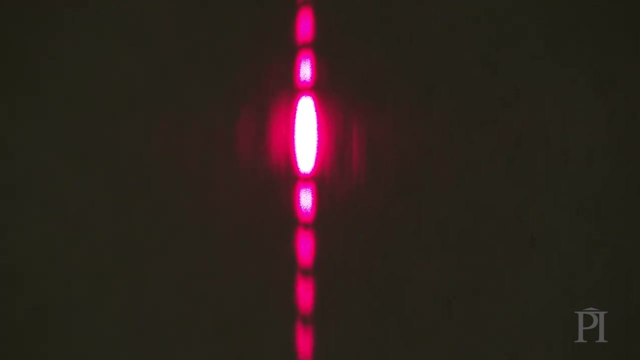 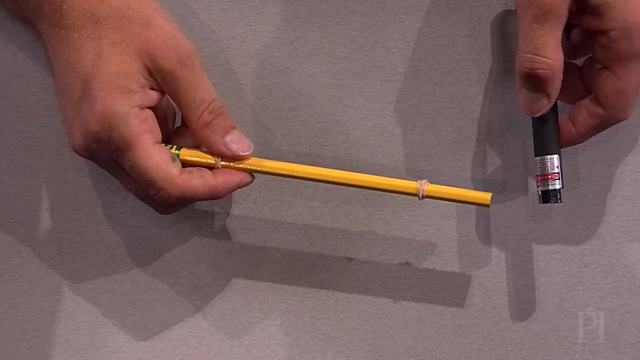 a table to make the pattern steadier. Now hold the pencils near the middle and gently squeeze them together. The central spot in the diffraction pattern gets taller. The more you squeeze, the taller it gets. To help students get more out of this demonstration, have them. 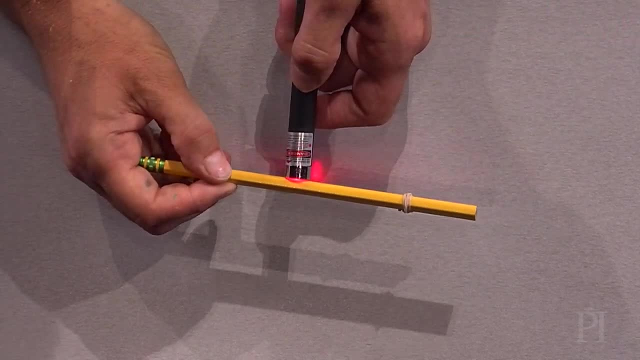 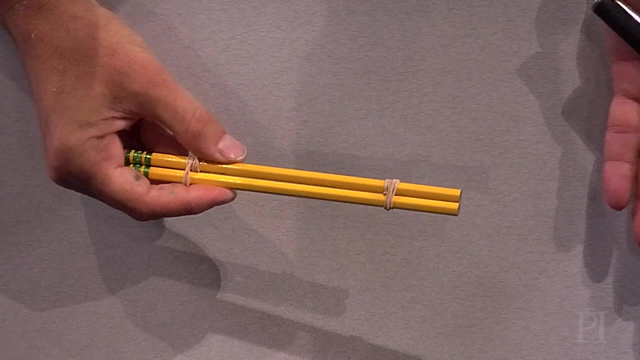 predict what will happen when you first shine the laser through the gap. Have them also predict what will happen when you squeeze the pencils. How does this show Heisenberg's Uncertainty Principle? This principle is all about trade-offs. If you don't know what to do with the pencil, you can use a pencil to. 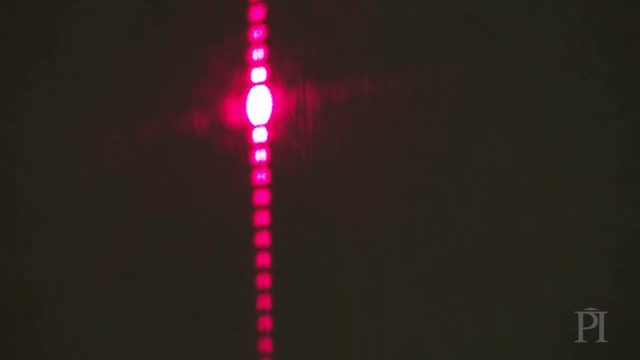 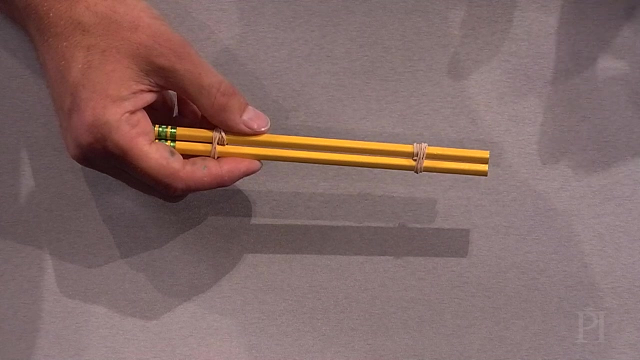 find out. The more you know about position, for example, the less that you can know about momentum. The size of the gap between the pencils is the uncertainty in the position of the photons making up the laser beam, And the height of the central spot is actually the uncertainty in the 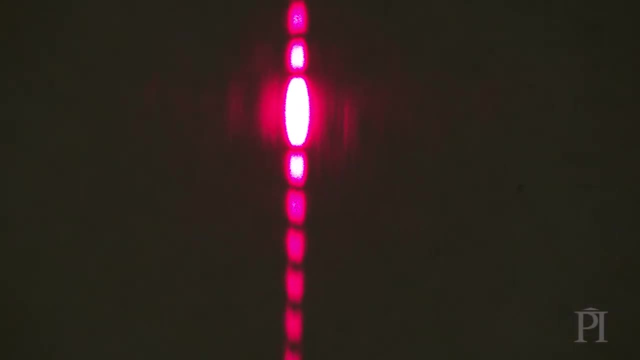 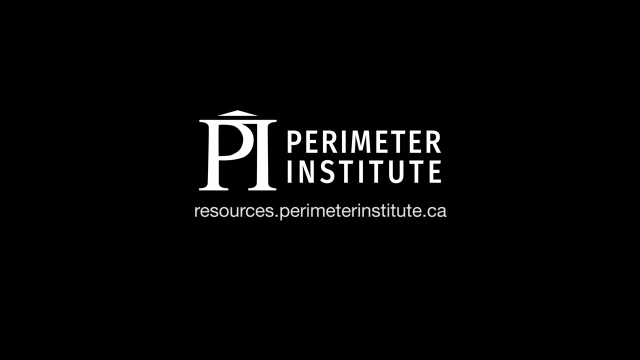 photon's momentum. The inverse relationship between these two quantities is an example of Heisenberg's Uncertainty Principle. Subtitles by the Amaraorg community.